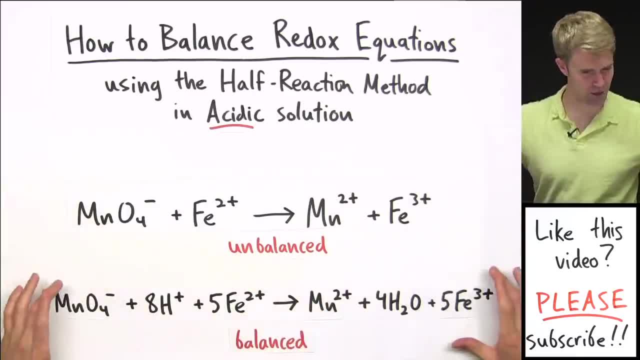 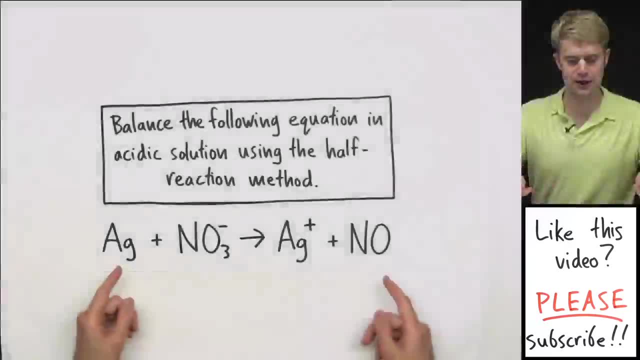 In this video we're going to look at how to balance redox equations using the half reaction method in acidic solution. Ready, Let's do it. Here's the equation that we're going to balance Now. balancing a redox equation is: 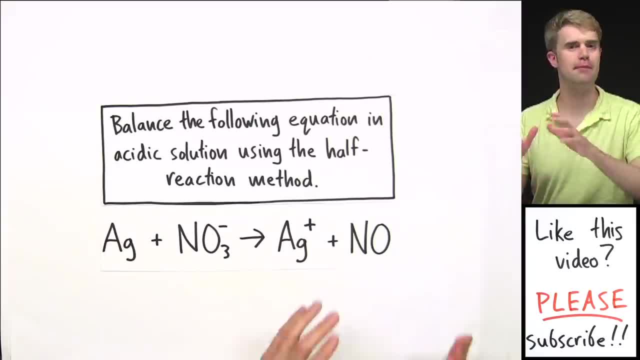 a little bit more challenging than just balancing a regular chemical equation, Because with a redox equation we have to balance not only the individual atoms but also the charges. So there's a step-by-step method we use that guides us through the process, kind of. 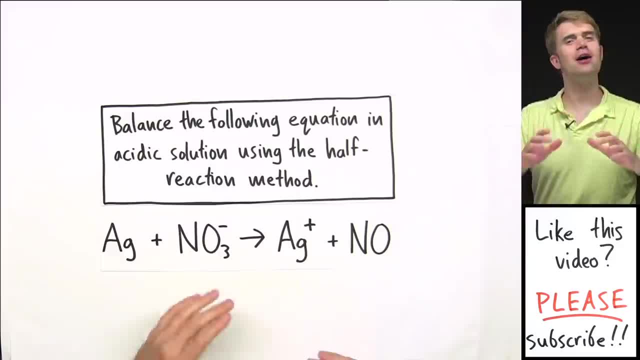 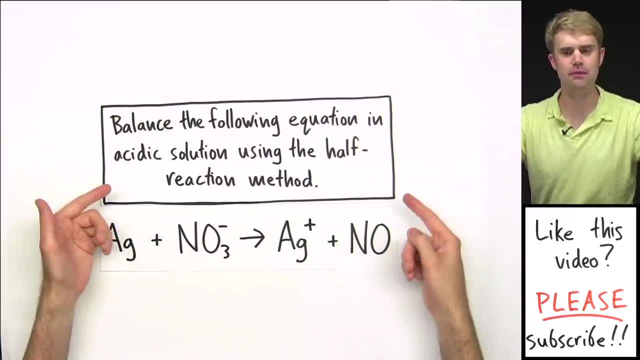 to make sure we don't forget anything along the way. I'm not going to talk about all the steps of this process right now. Instead, I'm going to introduce them one-by-one, as we use them while we work through balancing this example. So here's where we start. 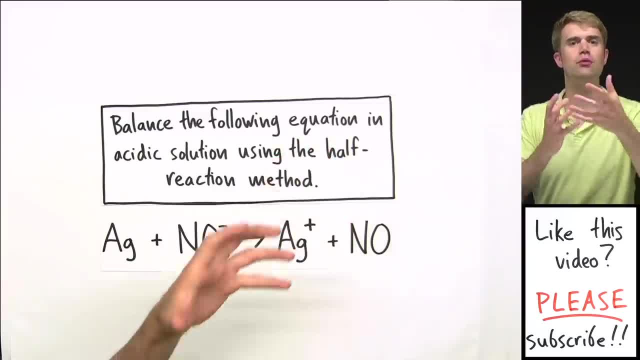 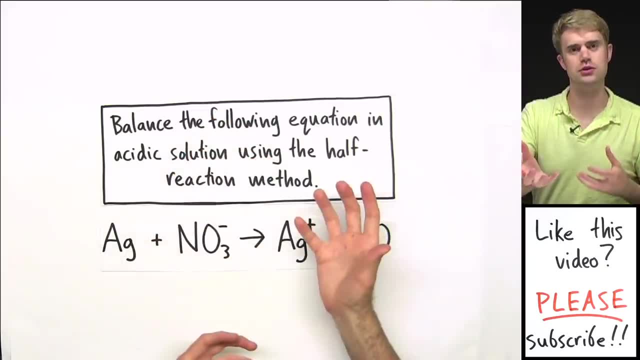 This is a redox equation, which means that there's oxidation and reduction going on. We want to know which else elements are getting oxidized and which are getting reduced. We can figure this out by looking at changes in the oxidation numbers for these elements. So the first thing we're 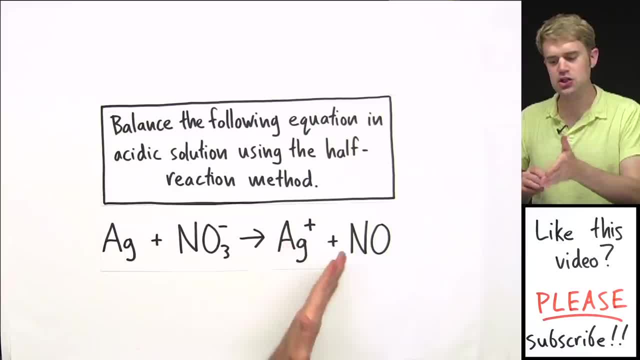 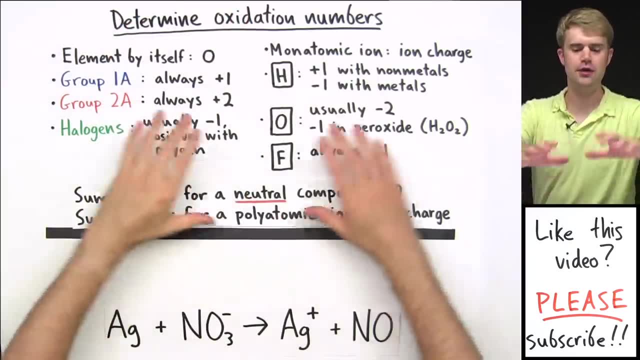 going to do is assign oxidation numbers to each of the atoms in this equation. So our first step is to determine oxidation numbers. These are the rules that we're going to use to figure out the oxidation numbers for the elements in this equation. Now, if this stuff? 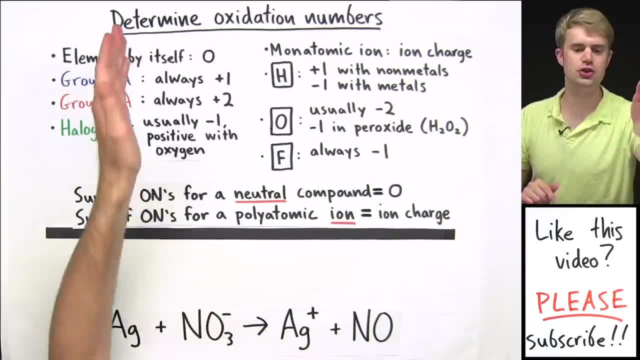 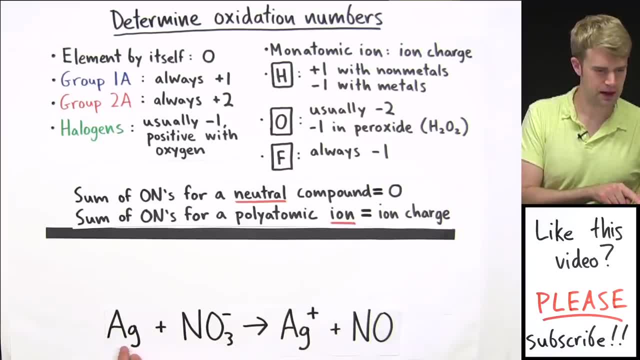 is totally new to you. I have a couple of things that I want you to know about. First of all, I have a couple of videos on just determining oxidation numbers. You might want to check that out for some background. Anyway, let's start with Ag, silver. here, Silver is an element. 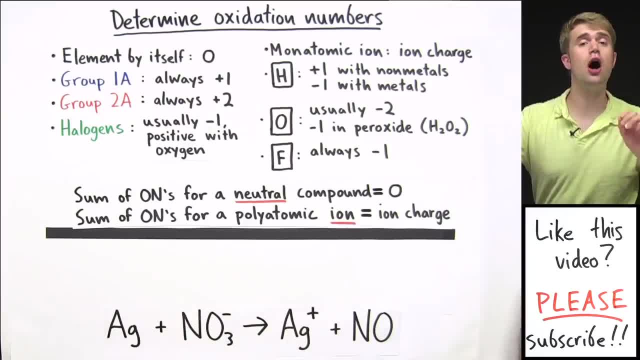 by itself. It's not combined with any other elements, It's just on its own, And so that means that its oxidation number is zero, NO3, one minus. here is a polyatomic ion. For N, for nitrogen, there's not a specific rule, so we'll have to figure it out. Oxygen is 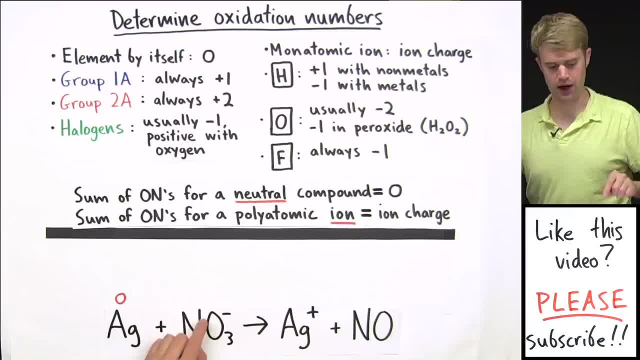 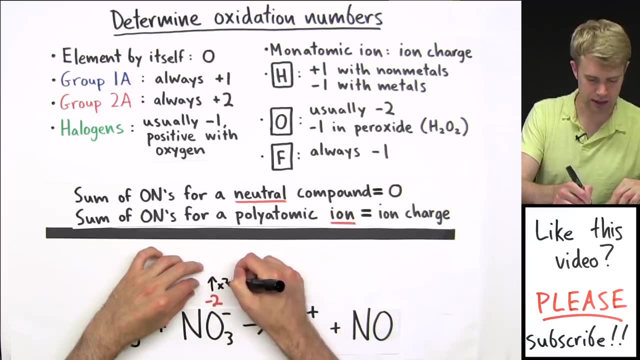 usually minus two, except minus one in peroxide. This definitely isn't peroxide here, So its oxidation number is minus two. Now in this compound there are three oxygens, O3.. So I'm going to multiply this negative two, this minus two times three, to get minus six. 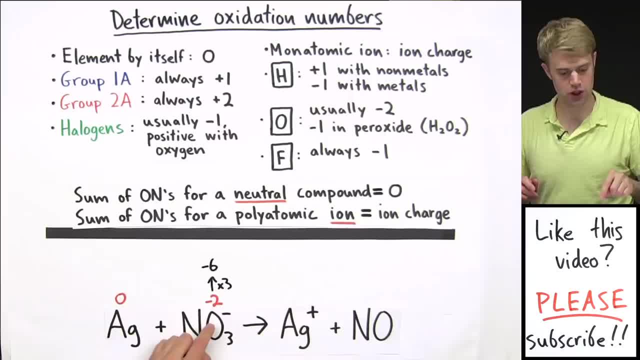 which is the total oxidation number for oxygen in this compound. Now to figure out nitrogen's. we're going to use this rule here that the sum of oxidation numbers for a polyatomic ion equals the ion charge. The ion charge here is one minus, and that means that whatever 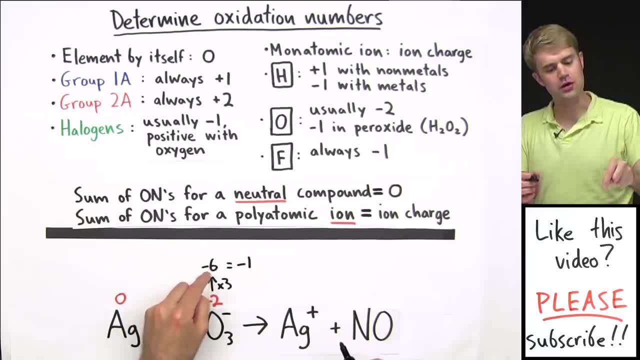 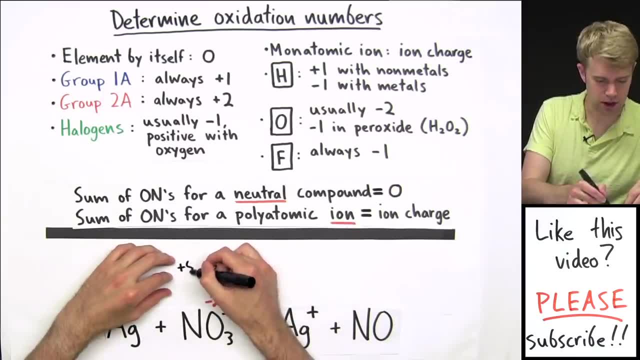 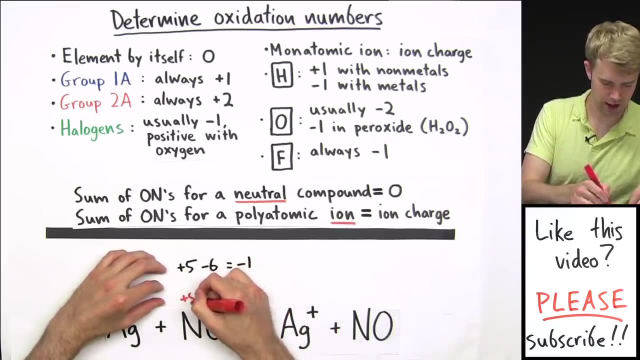 nitrogen's oxidation number is, when added with minus six, has to give us minus one. So that means that nitrogen's oxidation number is plus five plus five minus six equals minus one. So there we have it. Now let's look at oxidation numbers on this side of the equation. They're not. 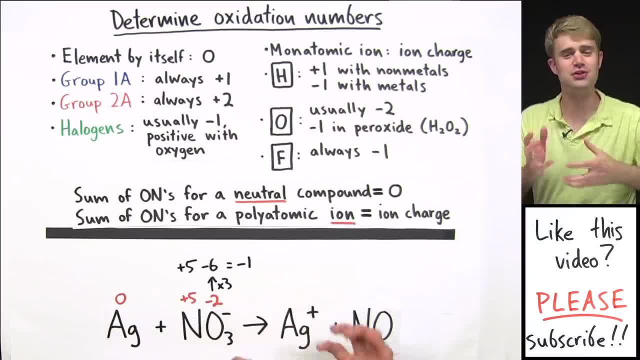 necessarily the same as they were over here, because oxidation numbers can change when the element is in different circumstances. So here Ag now has a charge of plus one. It's become an ion. it's become a monatomic ion made of just one atom. 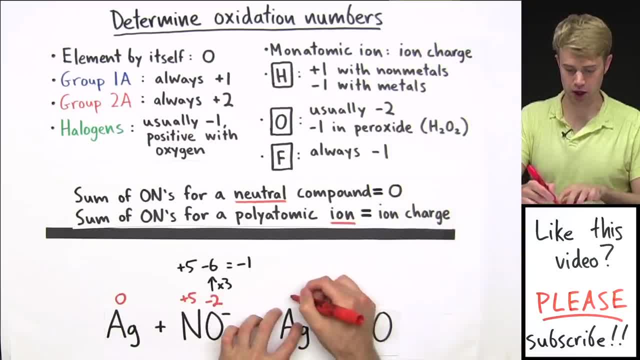 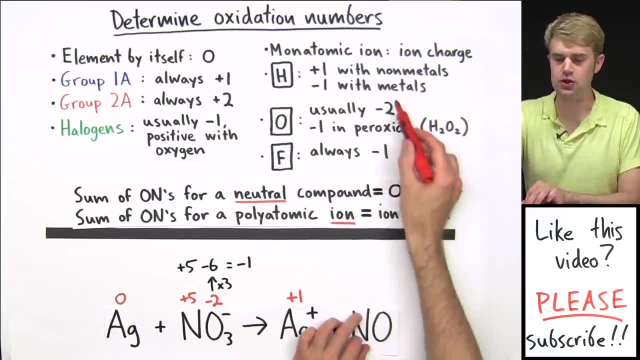 So its oxidation number is the same as its ion charge, So it's going to be plus 1.. And then over here we don't know nitrogen's oxidation number, but we do know that oxygen's is going to be minus 2.. 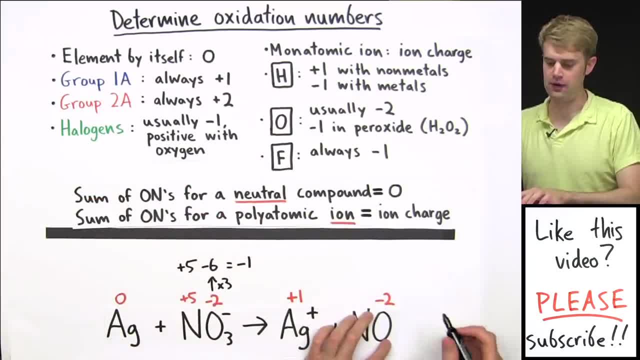 Then there's this rule here that for a neutral compound, the oxidation numbers have to add to 0.. NO is definitely a neutral compound because there's not a charge after it, which means that to add together with minus 2, you get 0.. 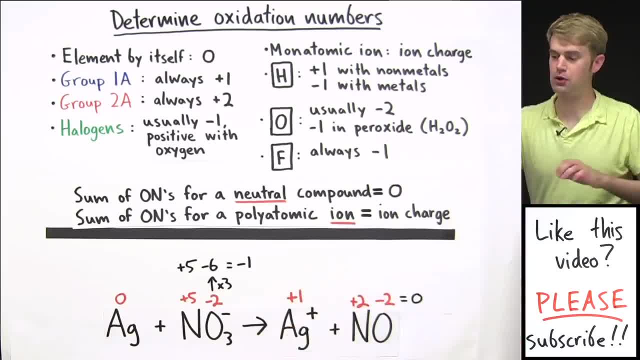 Nitrogen has to have an oxidation number of plus 2.. Plus 2 minus 2 equals 0. So these are the oxidation numbers for the elements in this equation. Now that we've determined these oxidation numbers, we can figure out what's being oxidized. 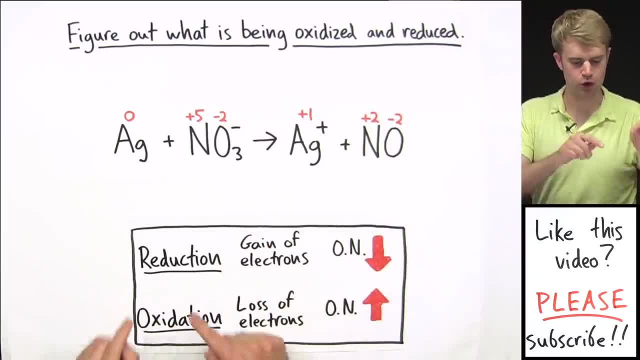 and what's being reduced. Take a look at this chart here. Reduction is a gain of electrons and it causes the oxidation number to go down. Oxidation is a loss. It's a loss of electrons and it causes the oxidation number. 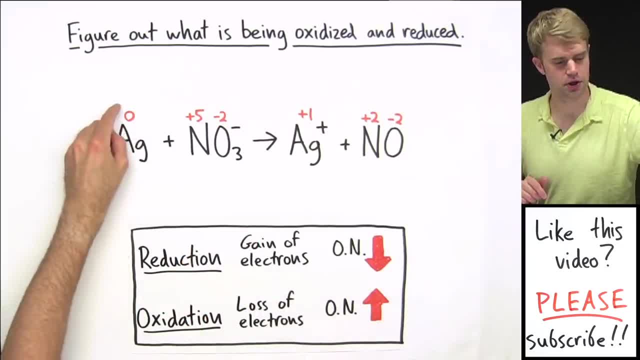 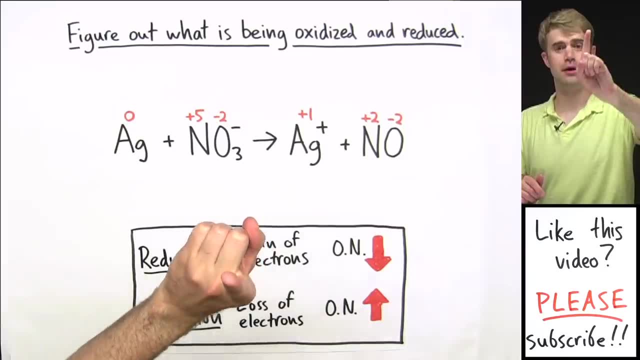 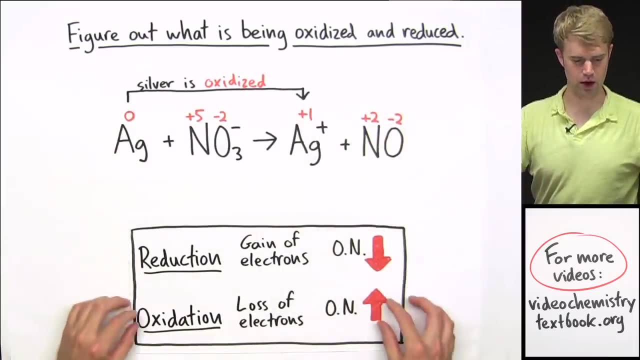 to go up. OK, Silver here starts out as 0 on this side of the equation, And then over here it becomes plus 1. So its oxidation number is going up, which means that it is being oxidized from 0 to plus 1.. 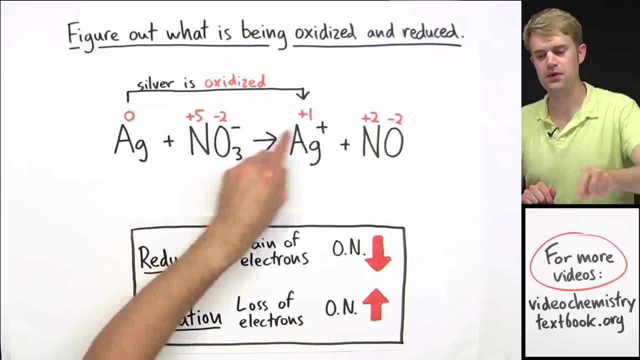 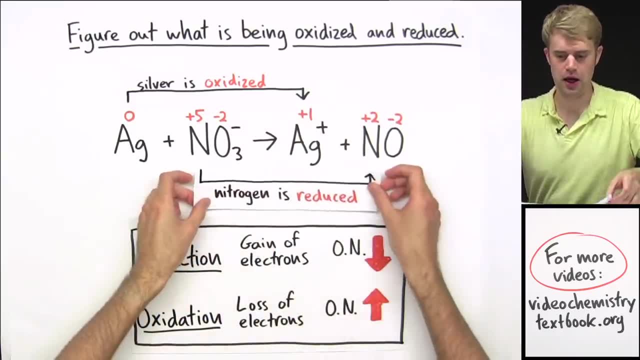 Nitrogen here is plus 5 over here, but then it's plus 2 on this other side of the equation, So its oxidation number is going down, Which means that nitrogen is being reduced. Now just let's take a look at oxygen real quick. 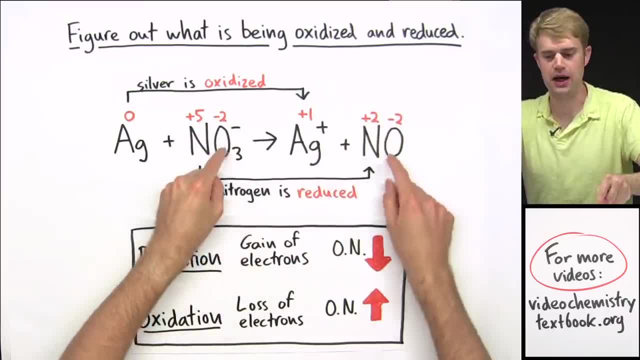 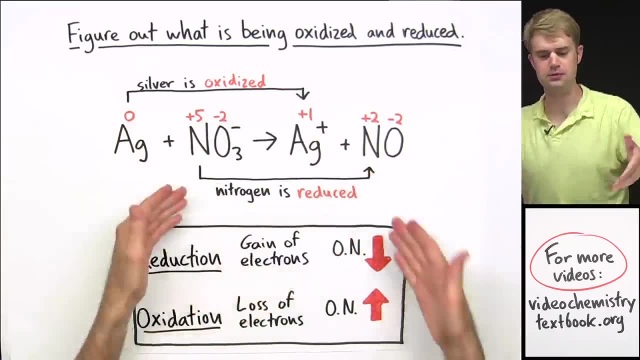 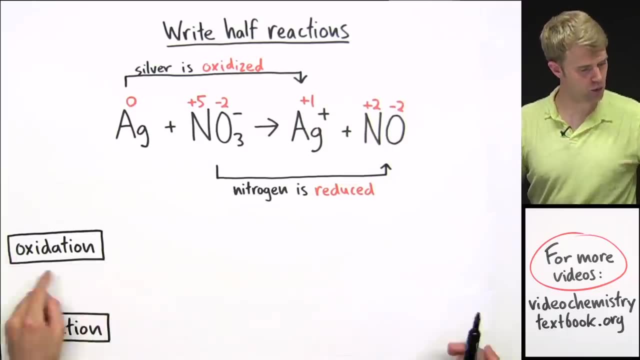 Oxygen is minus 2 here and it's minus 2 on this side, So nothing is happening to oxygen In this equation. silver is being oxidized and nitrogen is being reduced. Now we're going to write half reactions for the oxidation and for the reduction separately. 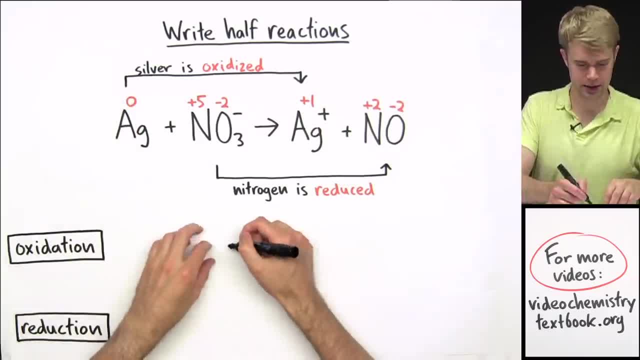 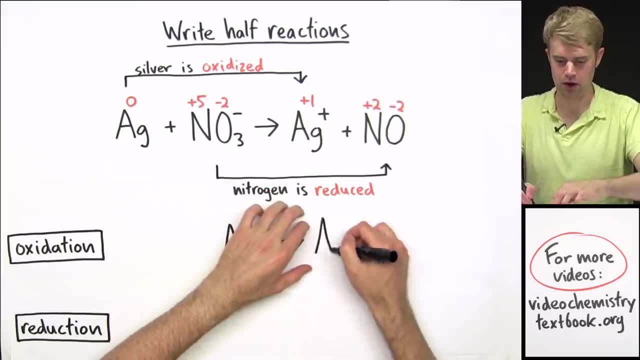 We'll start with the oxidation here. Silver, as we said, is getting oxidized, So we have Ag on one side of the equation And then we have Ag1 plus on the other side of the equation. This is the oxidation half reaction. 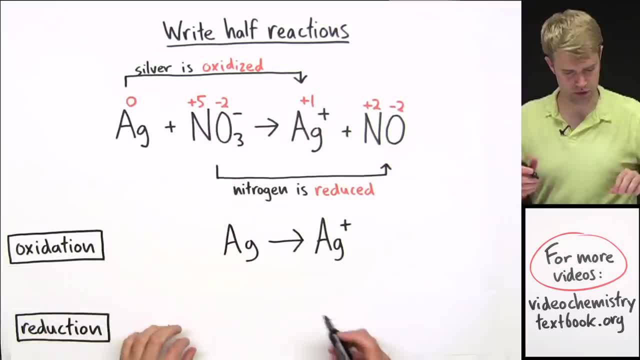 And now the reduction half reaction is going to be NO3 1 minus, NO3 1 minus, And then, on the other side of the equation, we're going to have NO. Now, the next thing that we're going to do is we're going to balance each one of these. 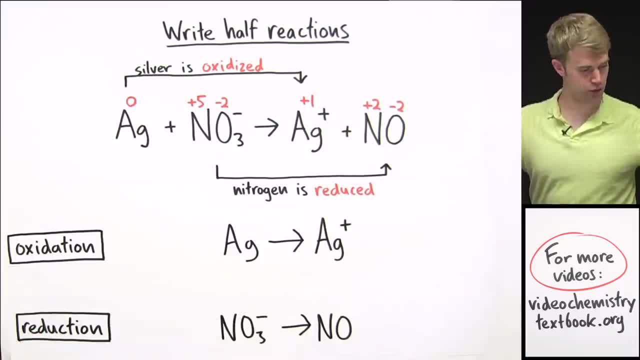 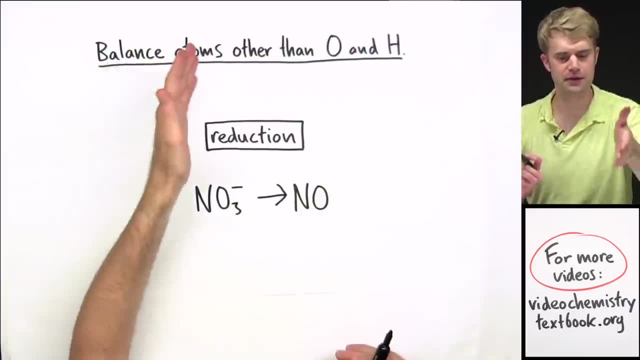 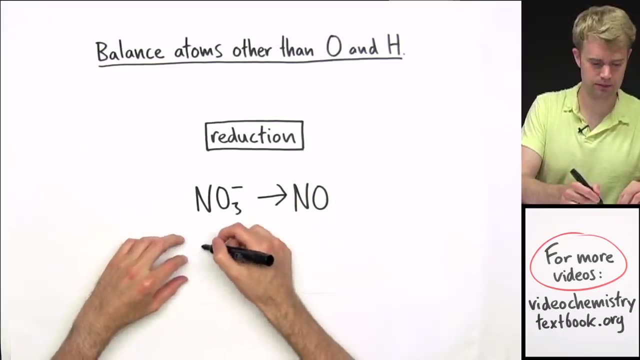 equations separately. I'll start with the equation for reduction and then we'll balance the equation for oxidation. Here's a reduction, half reaction. We're going to start by balancing the atoms other than O and H. Here's what that means. We have two elements in this equation. 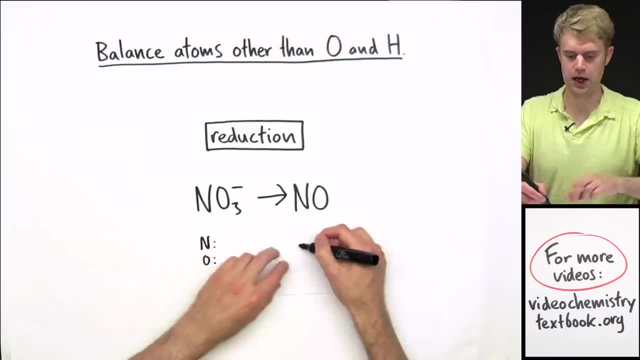 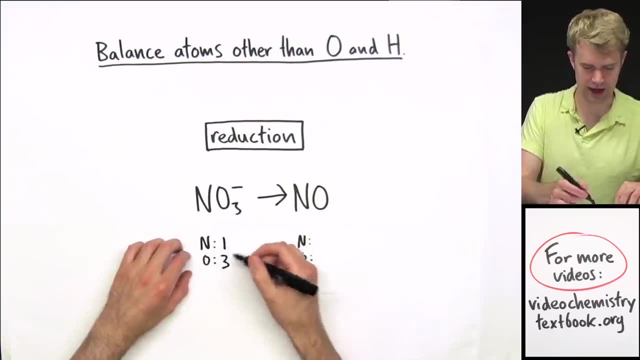 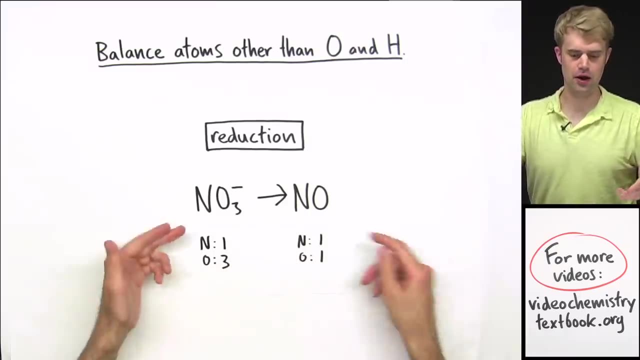 We have nitrogen and oxygen on both sides right here, On this side of the equation, we have one nitrogen and we have three oxygens- O3.. And on this side of the equation we have one nitrogen and one oxygen. So the nitrogen is balanced, one on both sides. 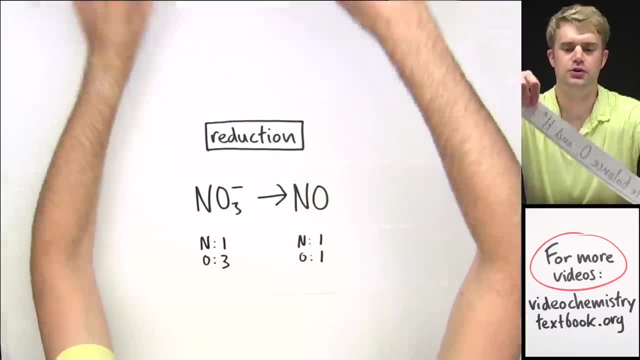 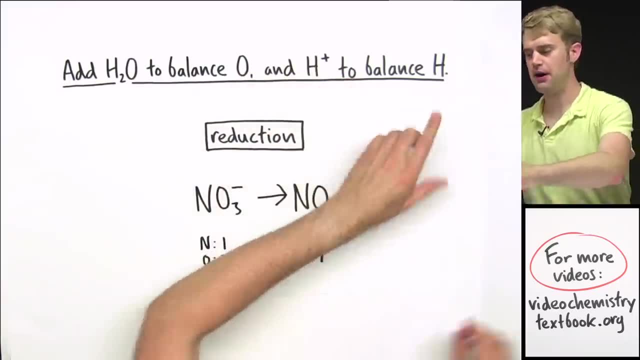 So we're ready to move on. The next thing that we're going to do is we are going to use H2O to balance oxygen and H plus to balance H. Here's what that means: We have an imbalance right now of oxygen. 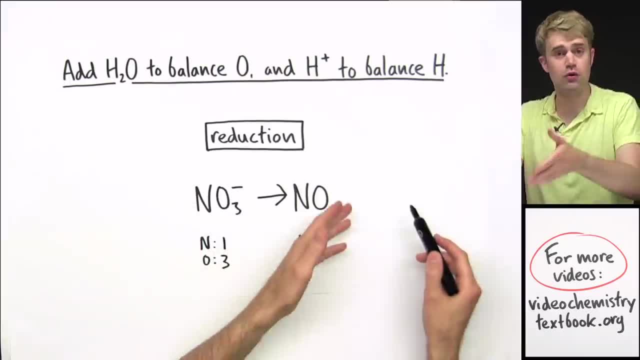 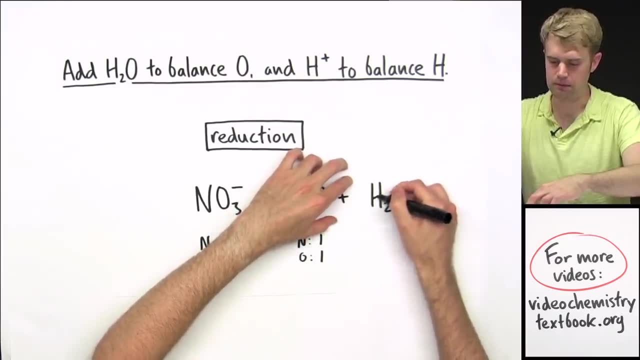 We have more oxygens on this side than on this side. In order for this to balance, we're going to add oxygen. We're going to add H2O, which provides oxygen. There is one oxygen atom in each H2O molecule. 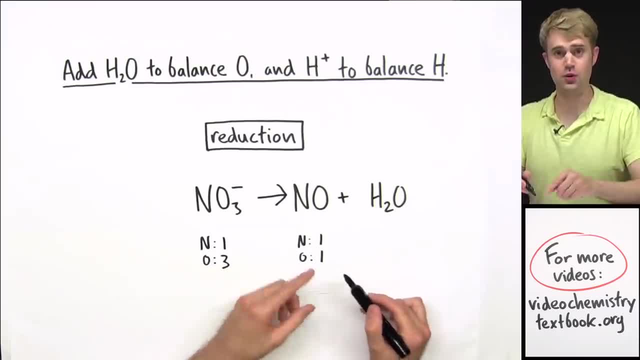 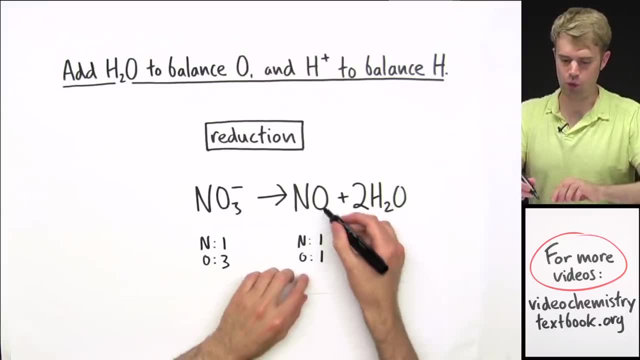 And I have three oxygens on this side, one on this side, So I need two more oxygens, So I'm going to put a two in front of this. So now I have one plus two oxygens, which gives me three oxygens. 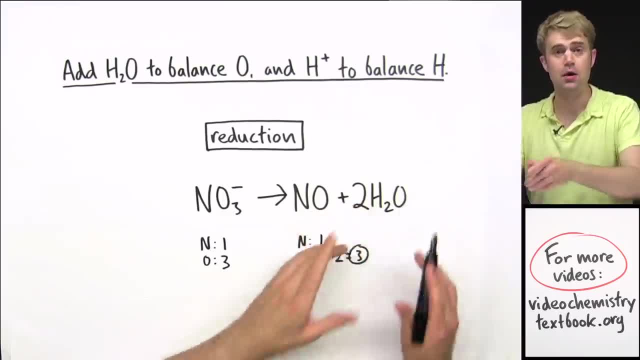 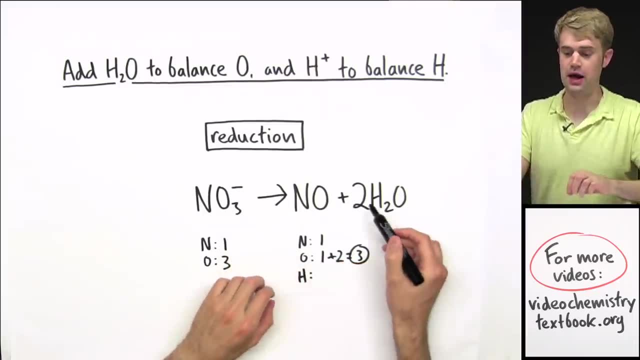 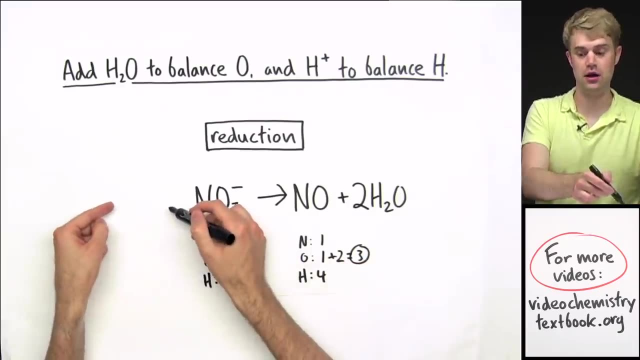 Now the oxygens balance by adding water. But I've introduced another element into the chemical equation, because now I have hydrogen And on this side I now have two times two, four hydrogens, And right now I don't have any hydrogens on this side. 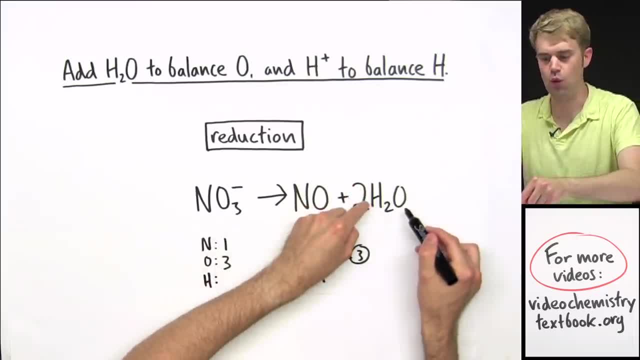 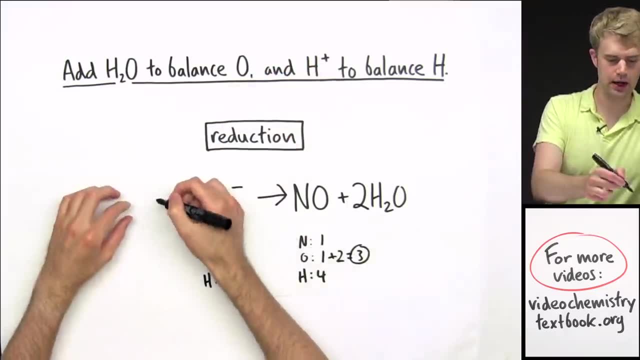 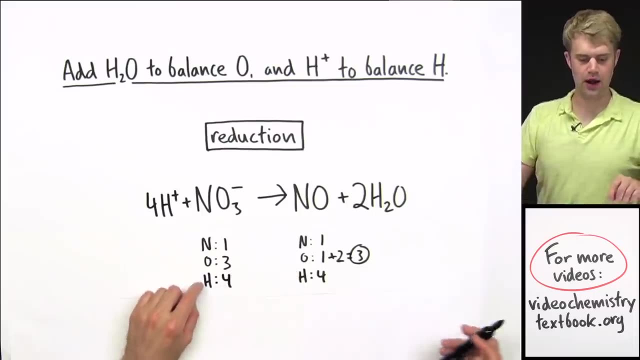 So, in order to balance out the hydrogens I added by introducing water, I'm going to add H plus to this other side. I've got four hydrogens on this side, so I'm going to add four H plus to this side. So now I have four hydrogens on both sides of the equation. 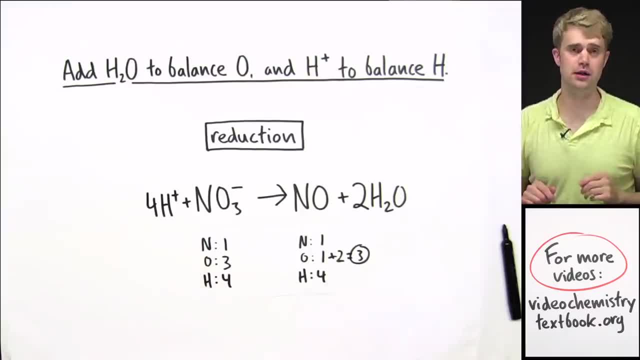 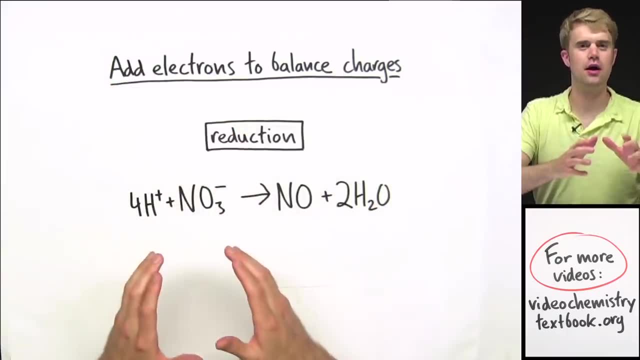 Now my nitrogens, oxygens and hydrogens are all balanced. Now that I've balanced the atoms in this equation, I now have to balance the charges by adding electrons. The concept of balancing charges in an equation might be new to you. 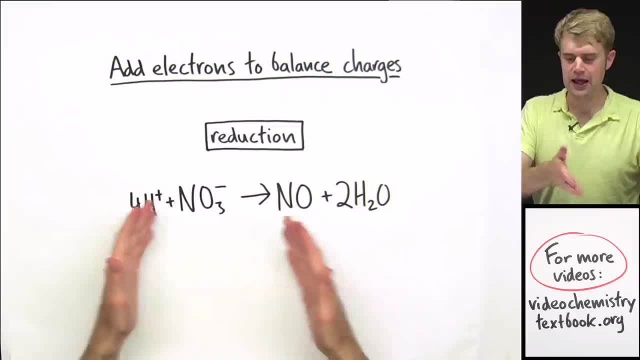 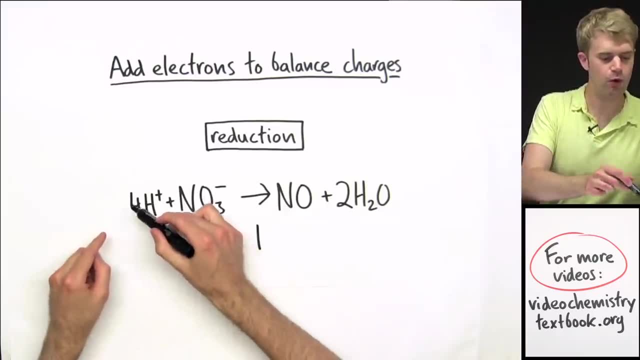 So let me walk you through this. The first thing I've got to do is determine how much charge I have on each side of the equation. I'll start over here. OK, I have four H plus. Each one of these H plus have a charge of plus one. 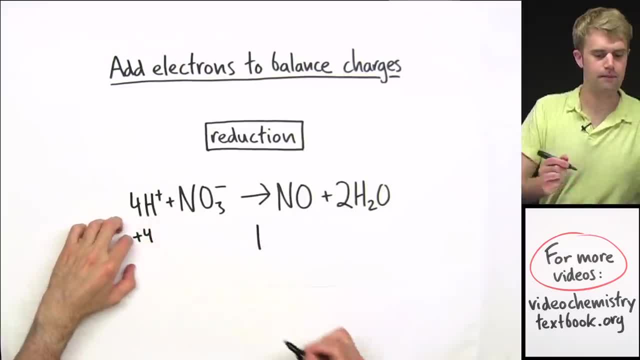 So four of those are going to give me plus four. Then I have one NO3 one minus with a minus one charge. So the total charge here I have is plus four from the hydrogens, minus one from the NO3. one minus gives me plus three. 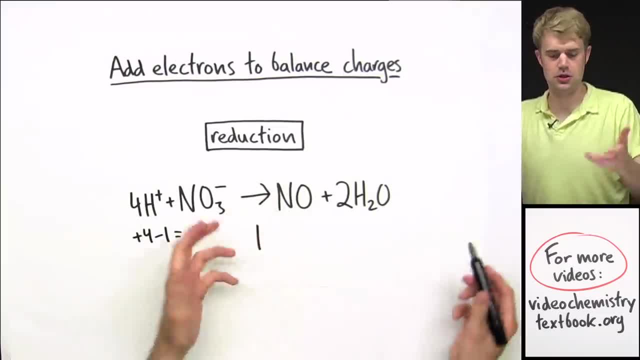 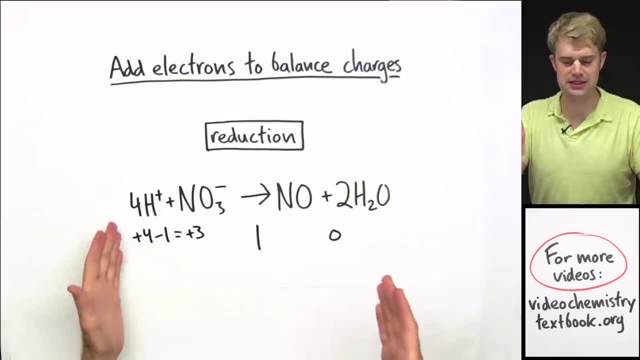 Now over here, on this side of the equation, I don't have anything that's charged, So the total charge here is going to be zero. That's simple enough. So now I've got to get these to balance. I need it to be the same charge number on both sides. 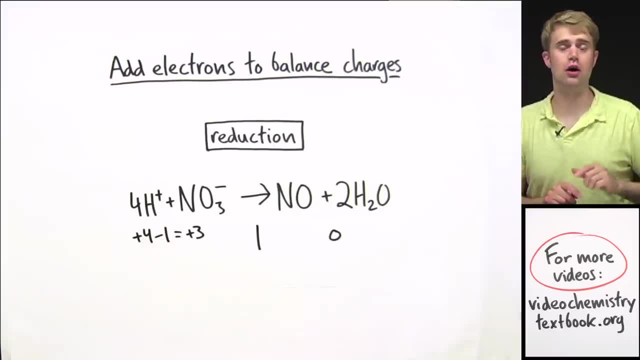 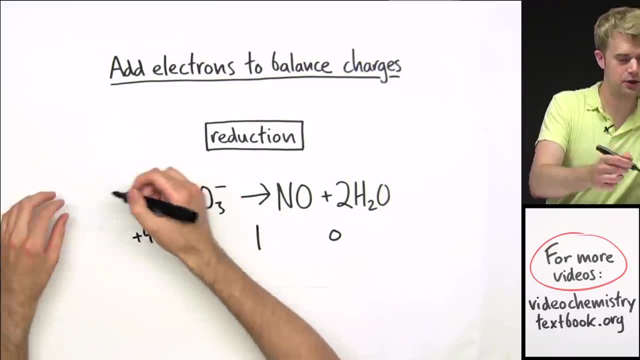 I need to find a way to cancel out this plus three of charge, And I'm going to do that by adding electrons, because electrons have a negative charge. So to this side of the equation I'm going to add three E minus the symbol for electron. 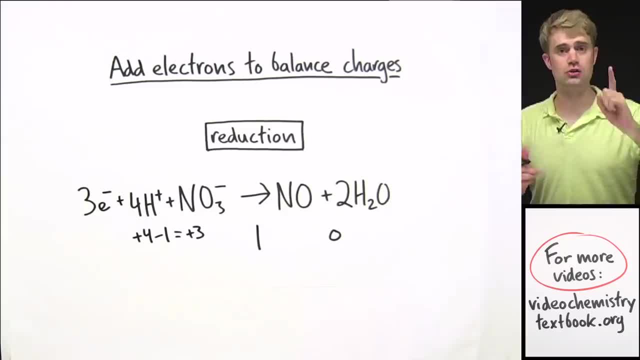 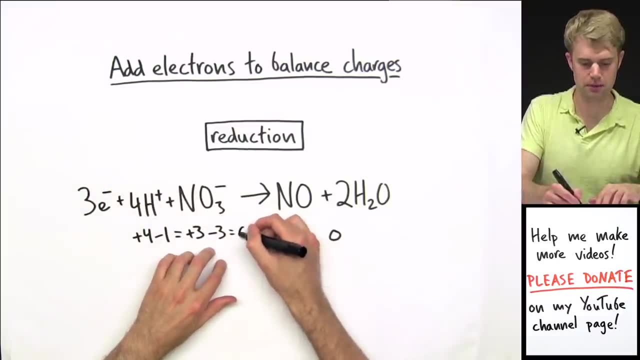 three electrons, each of which have a charge of one minus. So I'm going to have a negative charge. I'm going to have plus three minus three the charge from these electrons here, And that's going to give me a charge of zero. 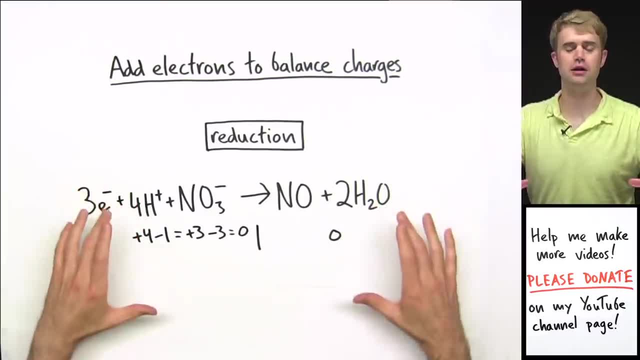 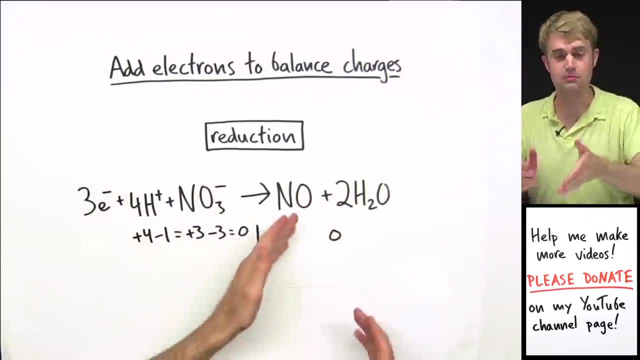 So now I've got zero on both sides of the equation and the charge is balanced. So the equation for reduction, or I should say the half reaction for reduction, is now balanced for atoms and for charge. Now I have to do the same balancing routine. 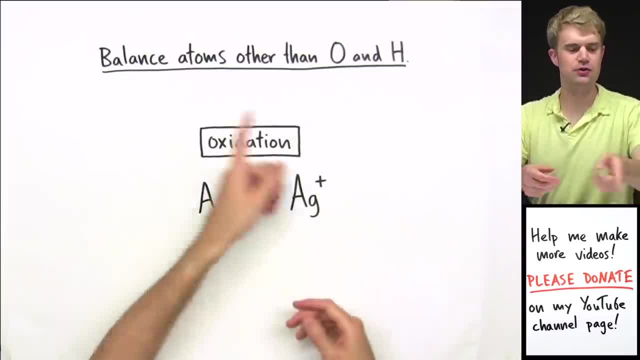 with the half reaction for oxidation. Here's a half reaction for oxidation. We have to balance the atoms other than oxygen, And I'm going to do that by adding oxygen and hydrogen. But we don't have to worry about that because we have one silver atom on this side. 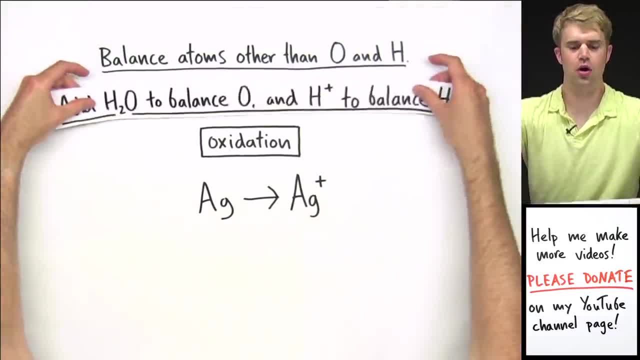 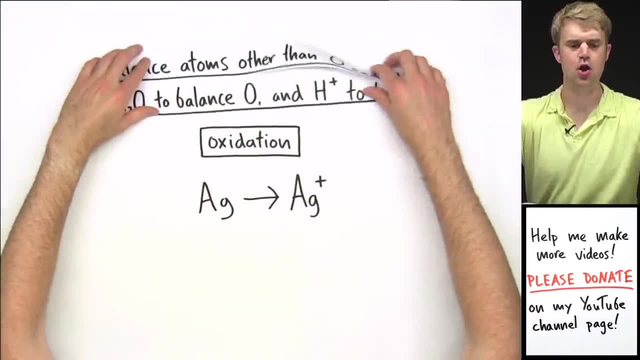 and one silver atom on this side, So it's already balanced. We also don't have to worry about adding water or H plus to balance out the O or H, because there are none of them in this equation, The only thing that we have to keep in mind. 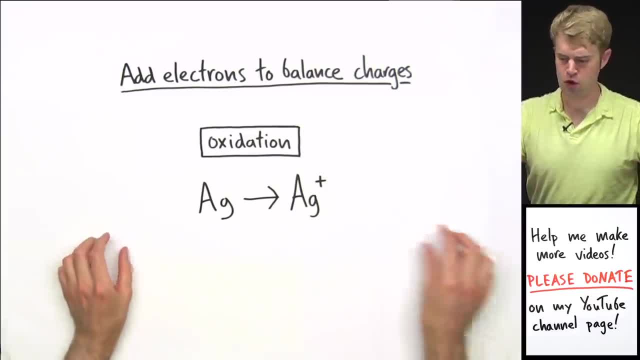 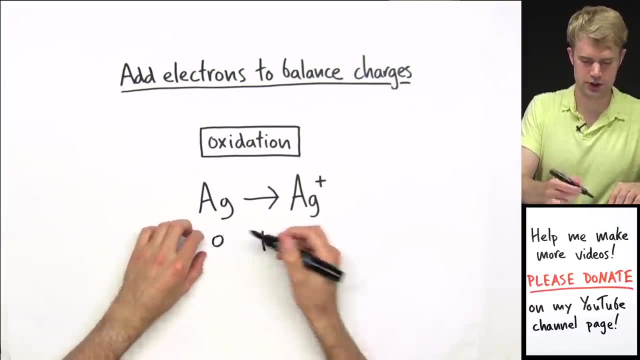 is the balance of the charges. Here's how we're going to do that. We're going to turn the charge on both sides of the equation: Over here, With no charge, so the charge is 0.. Over here, we have Ag1 plus, so the charge is plus 1.. 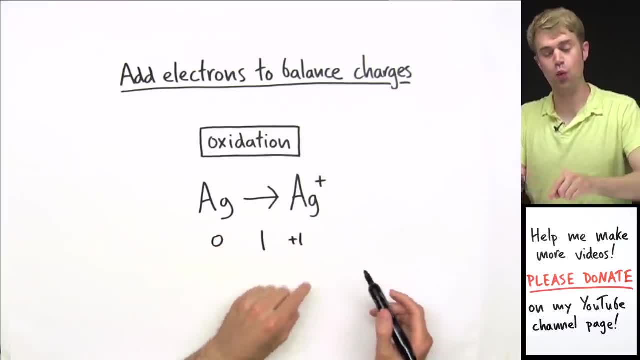 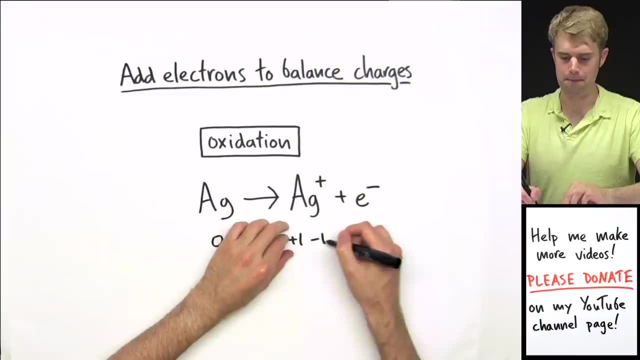 I need these charges to balance. So to cancel out this plus 1 charge, I'm going to add one electron with a 1 minus charge to this side. So now I've got plus 1, minus 1 equals 0, 0, 0. 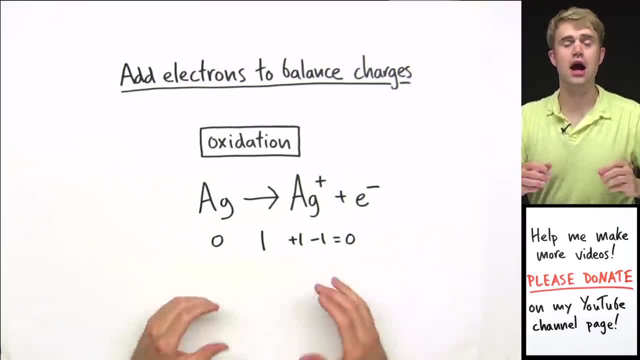 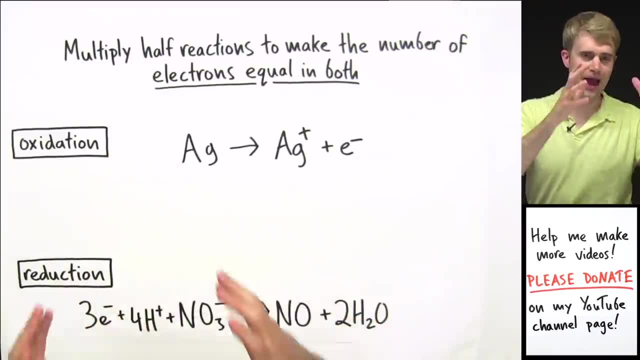 The charges balance. Now that I've balanced this, I'm ready to combine it with a half reaction for reduction. Now that I've balanced these two equations, for both atoms and charge, I'm going to start putting them back together. Let's look at the electrons here. 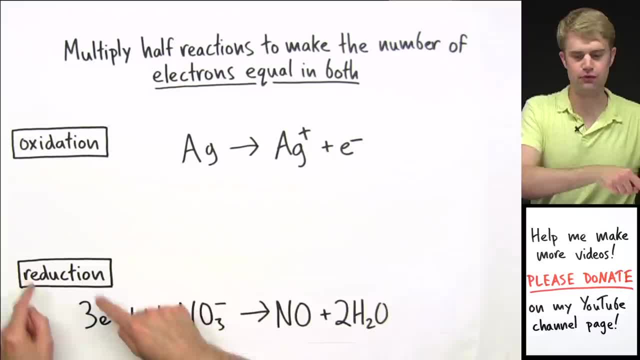 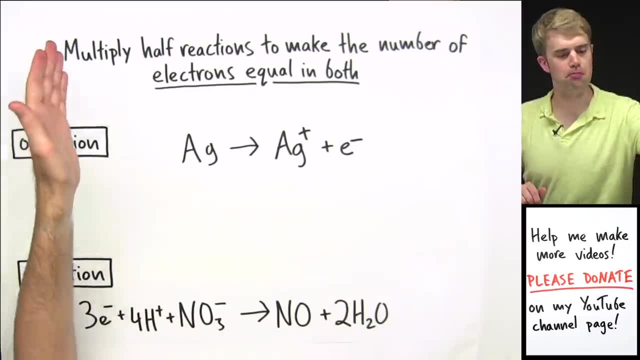 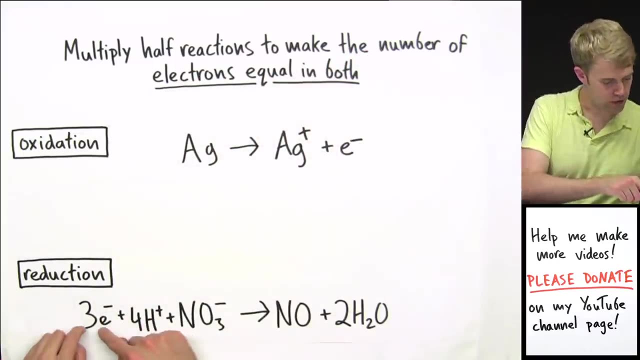 There are three electrons down here in the reduction half reaction And there is one electron here in the oxidation half reaction. What I want to do is multiply the half reactions to make the number of electrons equal in both, Since there are three electrons down here. 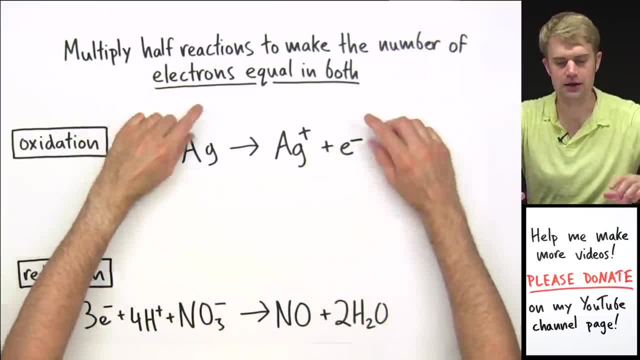 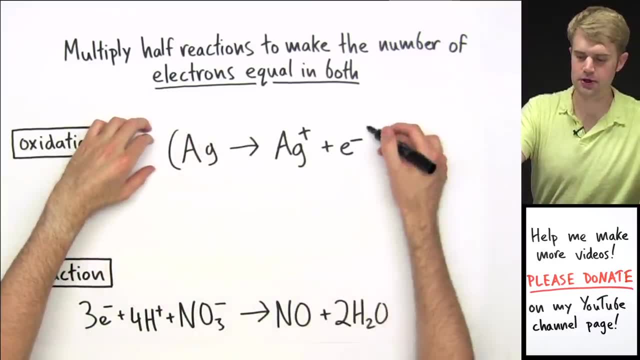 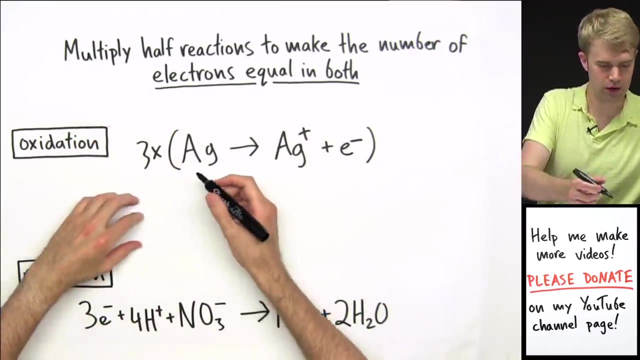 and one electron up here. I can multiply this one and this whole equation by 3 to end up with three electrons, so they'll be the same. So I'm going to do that just as if it's a math equation, And I'm going to distribute this 3 across the whole reaction. 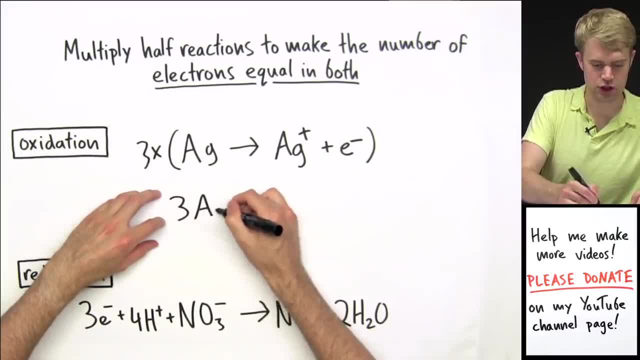 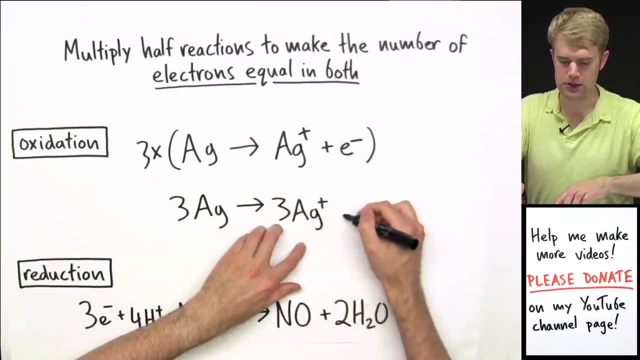 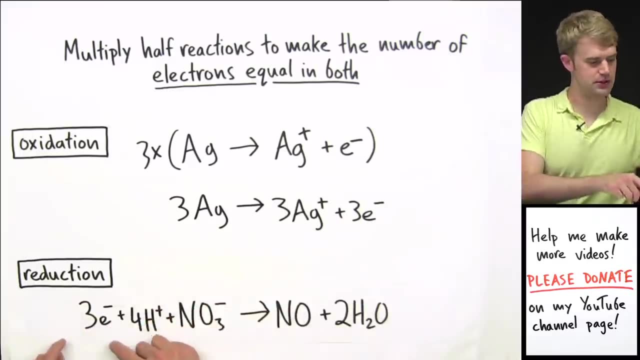 So that's going to give me 3 Ag on that side And then 3 Ag plus plus 3 E minus. Now the number of electrons balances in the reduction and oxidation reactions, Now that the number of electrons is the same in both reactions. 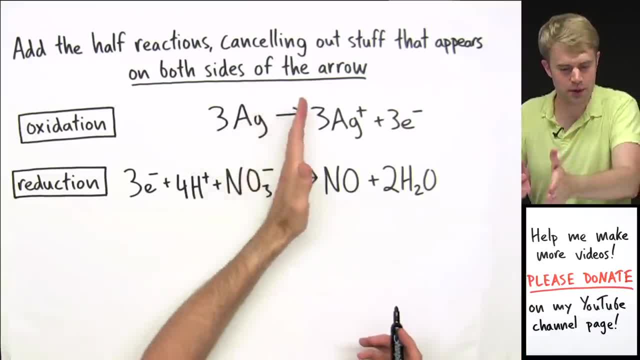 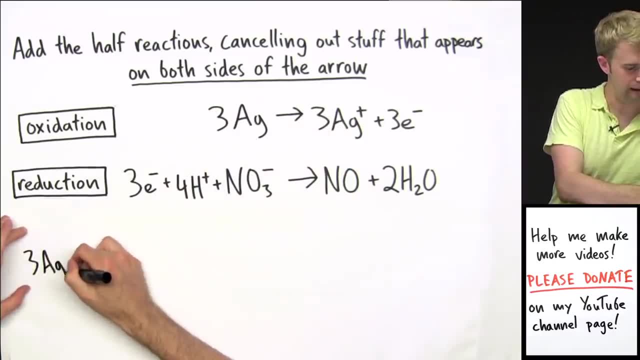 I can add them together. Let me show you how I do that. We'll start with everything on this side of the arrow. OK, I'll start with my 3 Ag, 3 Ag, And now I put in everything from this reaction. 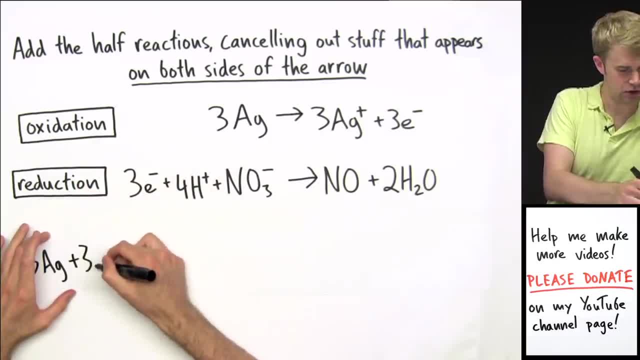 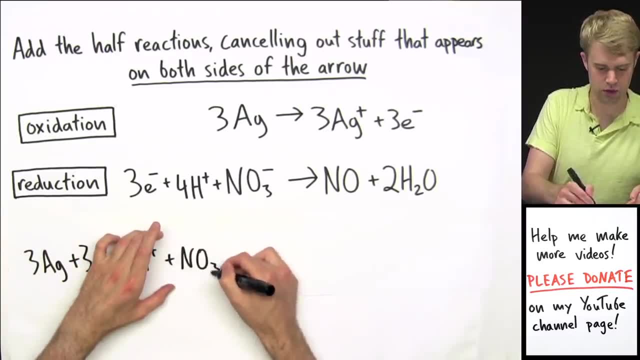 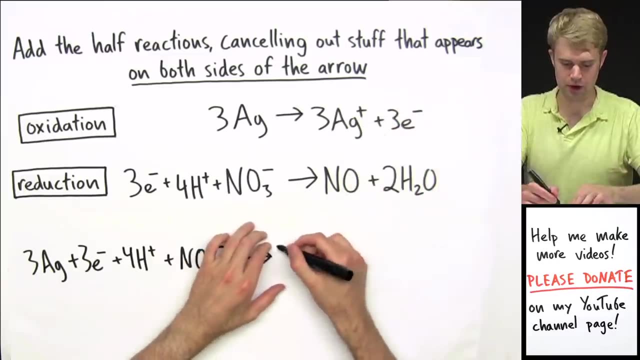 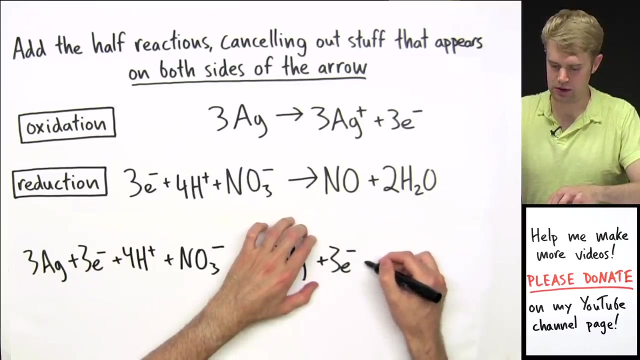 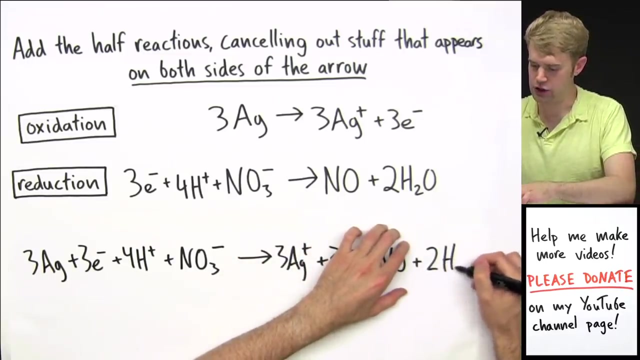 on this side of the arrow, 3 Ag plus 3 E minus Plus 4 H plus plus NO3, 1 minus. Then I put the arrow in And then I'll put in everything on this side I will have 3 Ag plus plus 3 E minus, plus this NO plus 2 H 2 O. 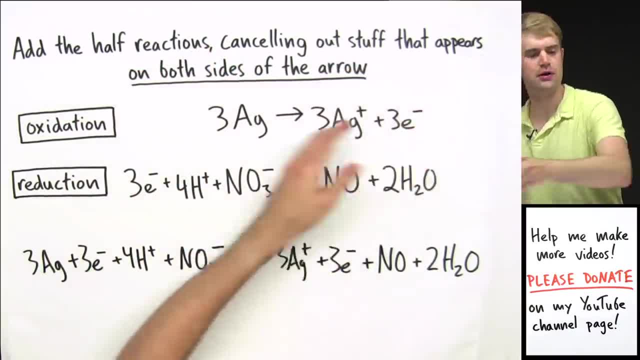 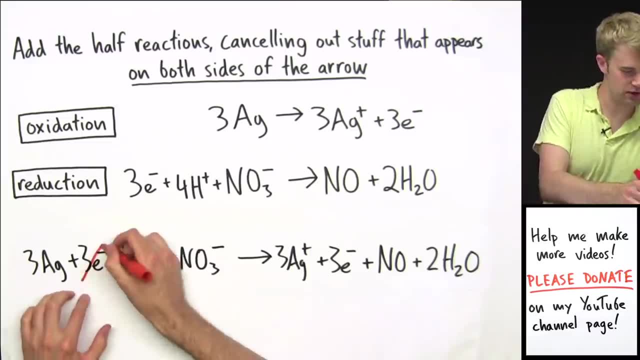 And now the next step up here says that we will be canceling out stuff that appears on both sides of the arrow. Let's look: We have 3 electrons on both sides of the arrow, So this can be canceled out, and this can be canceled out. 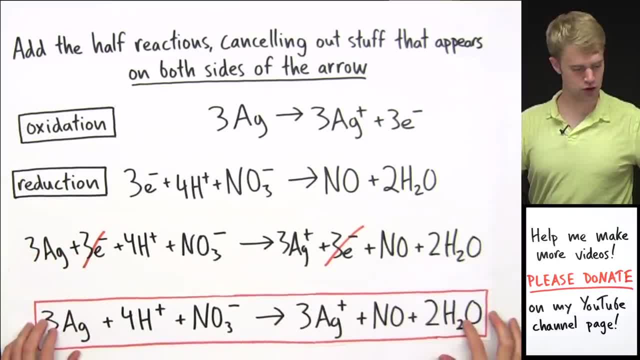 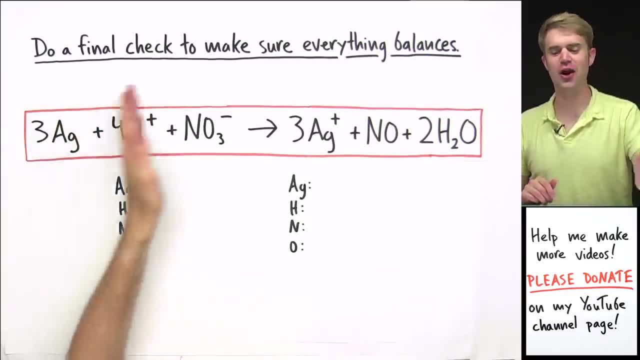 And when we rewrite this, after canceling out those electrons, this is going to be our final equation. Lastly, we'll do a final check to make sure everything balances here: The atoms and the charges. We'll start with the atoms, OK. 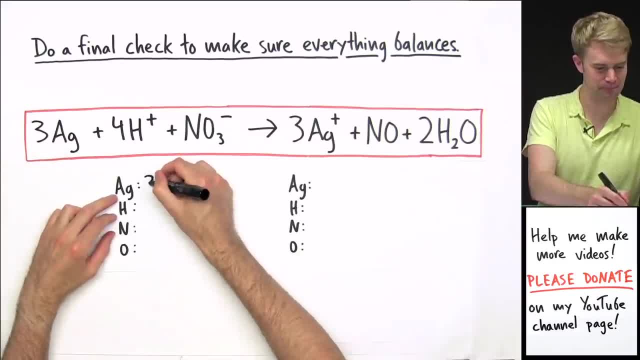 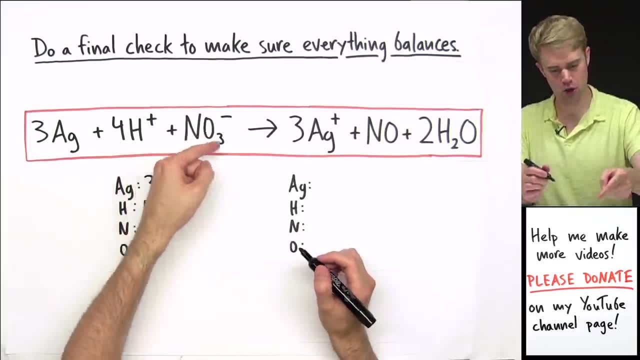 So we've got the atoms on this side, Ag, silver. we've got 3 of them: Hydrogens 4. Nitrogens just 1. And oxygen O3. We've got 3.. Over on the right side, silver Ag.